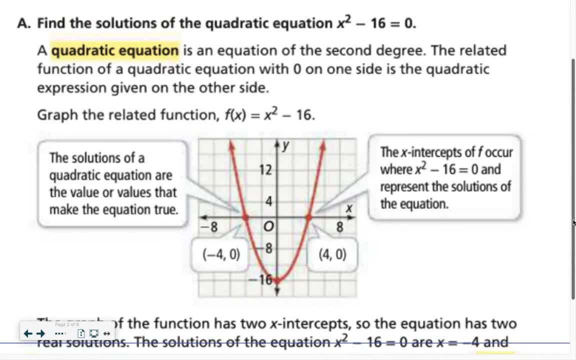 Okay, let's talk through this. I know there are a lot of words on the screen right now, So if we're finding the solutions, the solutions are the x-intercepts. Solutions of a quadratic equation are the x-intercepts. Sometimes there's two, sometimes there's one, sometimes there are none. okay, 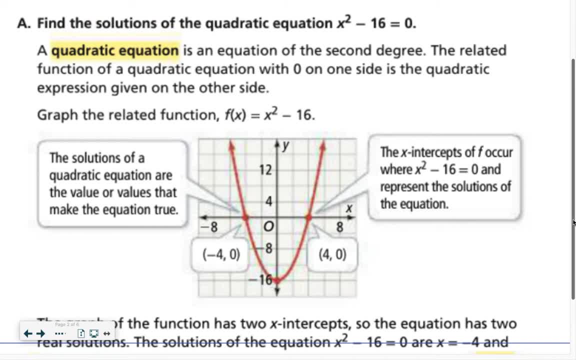 And so the way that you can tell how many solutions a graph has just by looking at it is: how many times does it cross the x-axis, And wherever it crosses, that is considered a solution. So if we look at this graph here, this is the graph of x squared minus 16.. 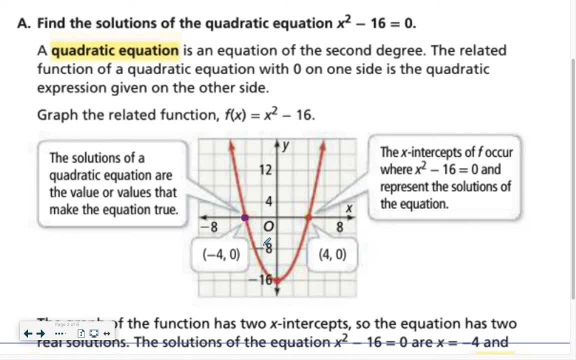 Okay, so you can see the graph crosses at a negative 4, 0 and a positive 4, 0.. Those are my two solutions, Okay, so if you're ever asked what are the solutions of a quadratic equation, it's wherever it crosses the x-axis. 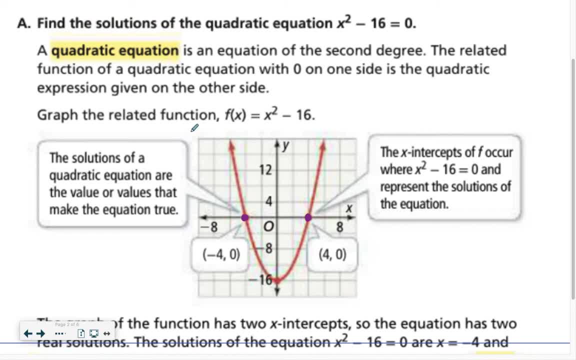 And for those of you that are like I, still don't understand what a quadratic equation is: just a couple of big words. well, refresh your course. A quadratic equation is an equation of the second degree. That means a quadratic equation has to have an x squared. 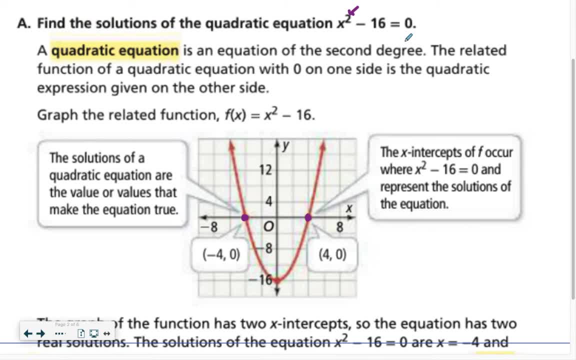 or whatever the variable is. squared term: okay. Quadratic is when you have that second power somewhere, that second degree, okay. And then when you hear the phrase related function of a quadratic equation with 0 on one side and the quadratic expression given on the other side, 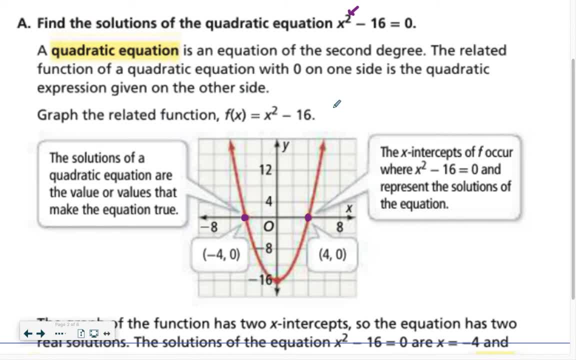 again. that's a lot of big words that you're probably like Ms Johnson. what is it saying? Yeah, this is the related function. Instead of it being equal to 0, they replace it with f of x. That's what all of this, all of these words, mean, okay. 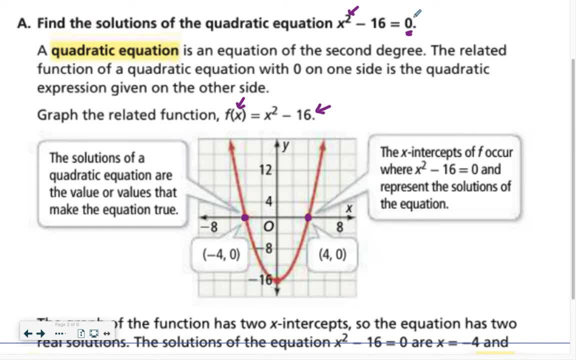 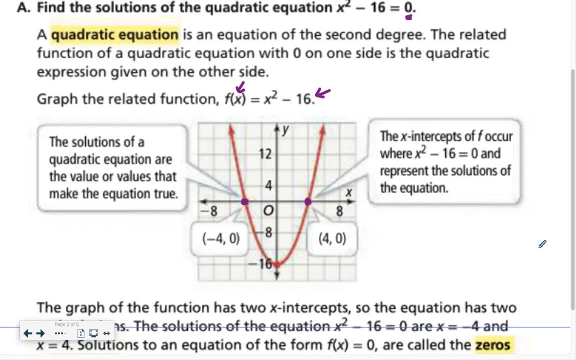 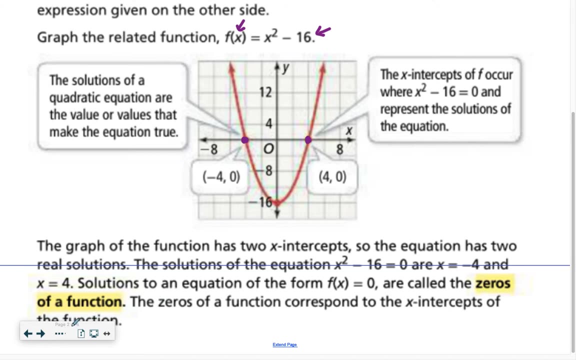 Related function: f of x equals. Equation 0 equals. okay, All right, so that is really the main takeaways here. okay, And the last thing that I'll share with you is that solutions are sometimes called the zeros of the function. 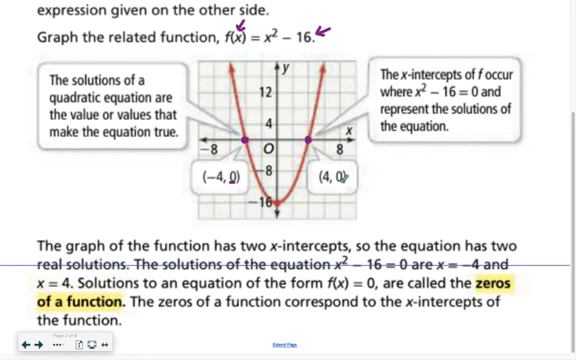 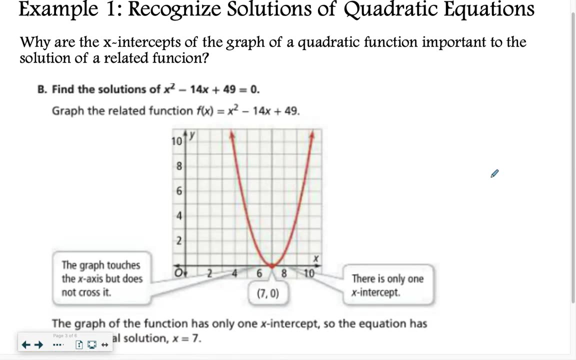 and that's because they give you 0 for y. okay, So solution is the same thing as zeros of of a function. okay, Then let's look at letter b. So this time you can see we have find solutions of x squared minus 14x plus 49 equals 0.. 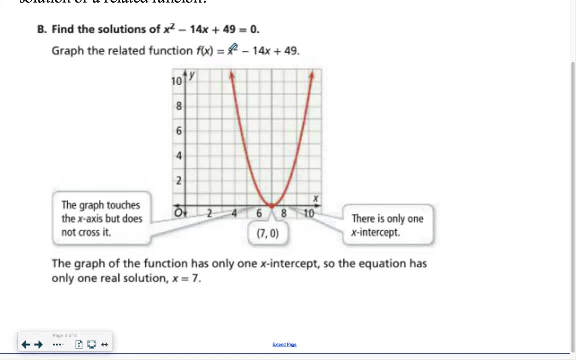 So you graph the function, which is: f of x equals x squared minus 14x plus 49.. It's a related function because it says f of x instead of 0 equals okay, Yada, yada, same thing, Um, but 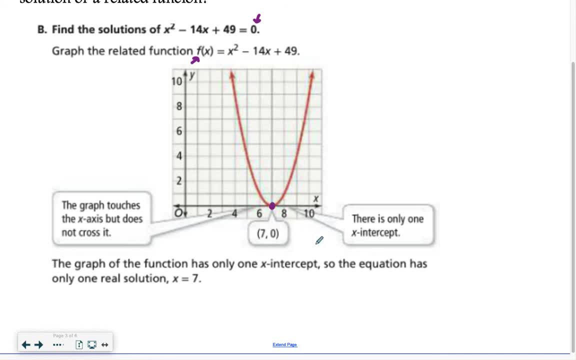 our solution here. you can see it only crosses the x-axis once. And some of you are gonna say, technically it doesn't cross because you like to. you know, look at the technicalities And you're right, it doesn't cross. 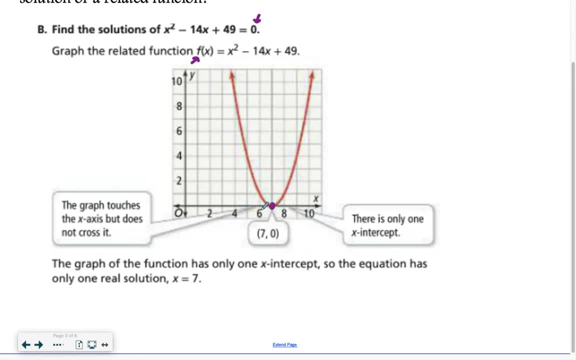 It doesn't go below the x-axis. It hits the x-axis and then stops. So intersect means it just has to touch it, okay. It doesn't have to go all the way through onto the other side, It just has to touch it. 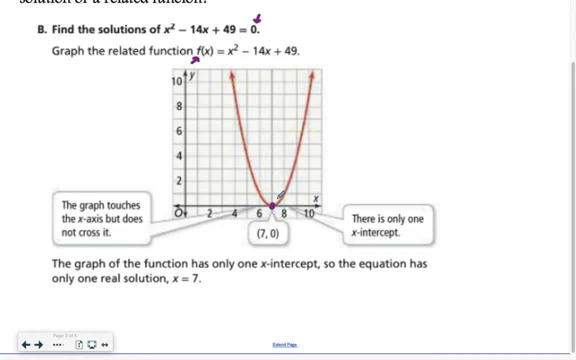 So this graph, this parabola, has one solution, and that solution is 7, 0.. So my 0 of the function is 7.. Or my one solution is x equals 7.. Or you can list it as 7 comma 0, the ordered pair. 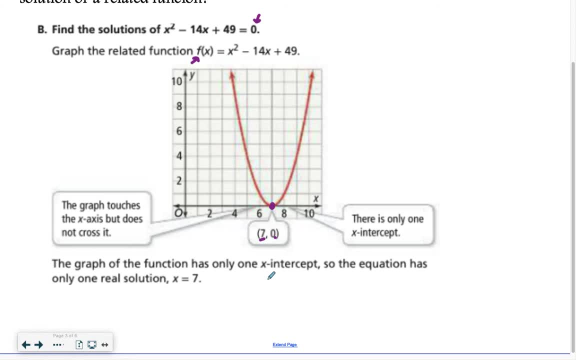 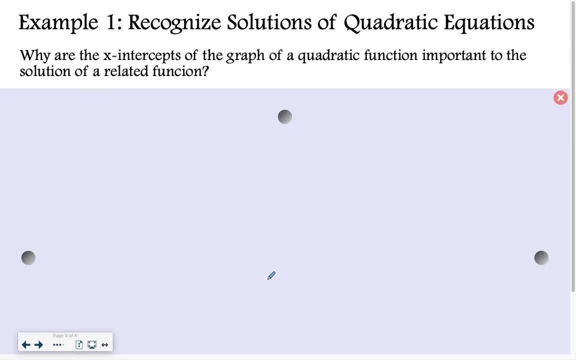 All of those are ways of telling a person what the solution is for the graph. It tells us where it crosses or hits the x-axis. All right, so we've done. we've. I've shown you a 2, solution. I've shown you a 1, solution. 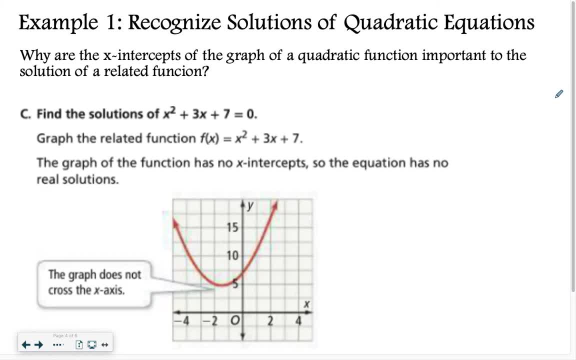 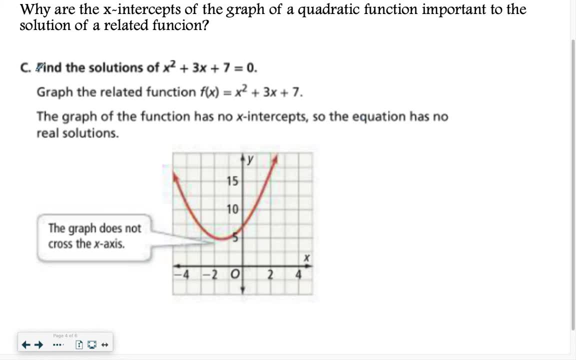 I wonder what. this will be. No solution. yay, Okay, can you tell I'm a little tired and slap happy right now. My apologies, All right. letter C: Find the solutions of x squared plus 3x plus 7 equals 0.. 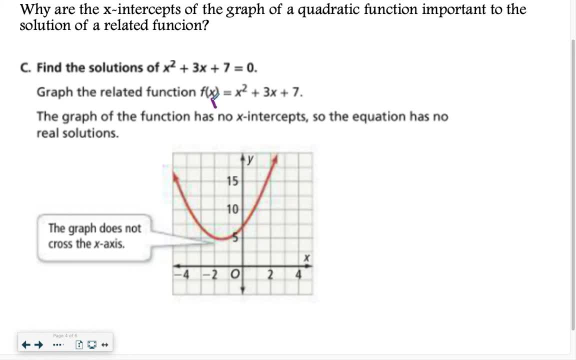 So first of all, graph the related function. Again, the related function just means we have f of x equals instead of 0 equals. I know I'm being really annoying by saying that on every single slide, but hopefully that means that the annoyingness 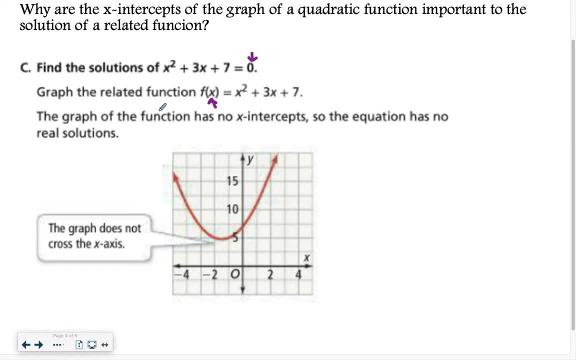 will help that information stick in your brains, okay? So graph the function x squared plus 3x plus 7, and you can see. this is what the graph looks like. This graph never, ever, touches that x-axis, So there are no solutions. 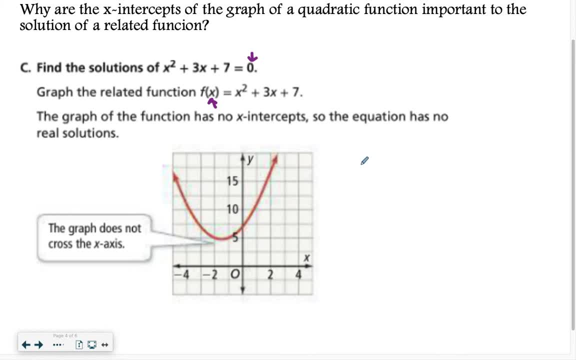 or your book is gonna be a little more technical, and they're not just gonna say no solutions, they're gonna say no, no solutions, Real solutions. And the reason they're gonna say no real solutions is because when you get to algebra two in a couple of years, 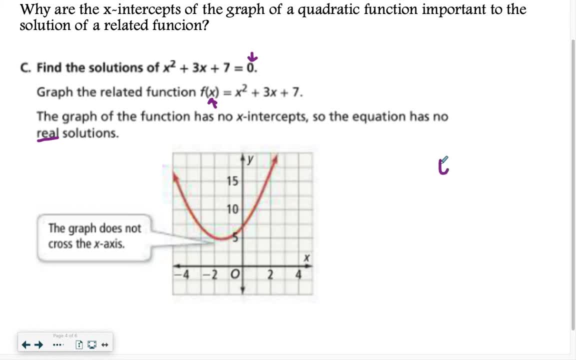 you're gonna learn about something called an imaginary number. Fun fact, it has a little i with it to represent that it's an imaginary number, But alas, you are in algebra one and we are not gonna deal with imaginary solutions right now. okay, 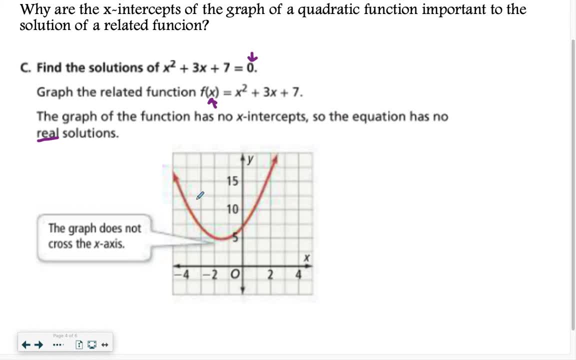 So you get to stick with just no real solutions. whenever it doesn't hit the x-axis, A common error I see students make is if it doesn't hit the x-axis, they will overcompensate and tell me where it hits the y-axis instead. 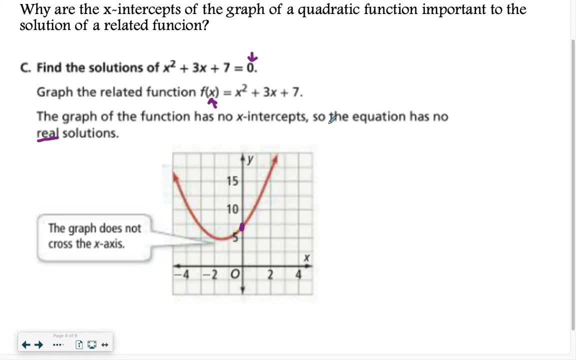 But honestly, I don't care where it hits the y-axis, I only care for solutions where it hits the x-axis. So you would need to say no real solutions here. And if you're asking me, do I really have to say no real solutions? 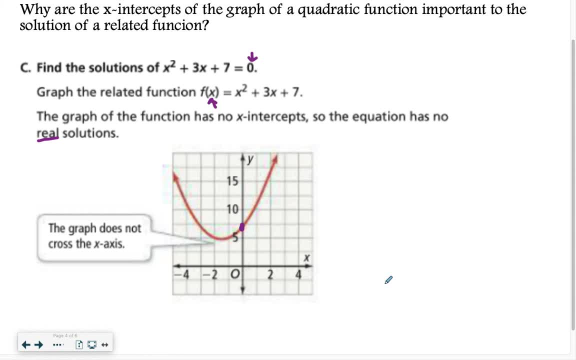 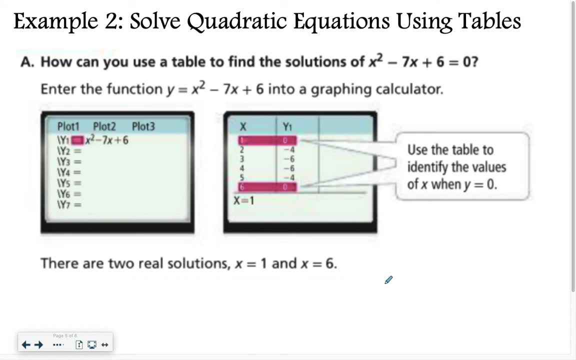 or can I say no solutions? The answer is yes. You really have to say no real solutions, All right. example two: solve quadratic equations using tables. We're not gonna get super into this because you don't have graphing calculators. 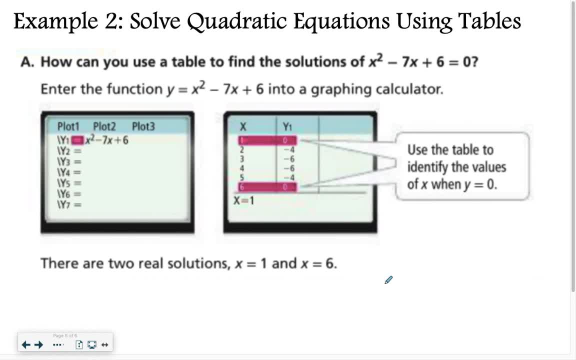 as I mentioned at the beginning of the video. But I want you to know how to tell what solutions are just by looking at a table. So how can you use a table to find solutions of x squared minus seven? Well, you can use a table to find solutions. 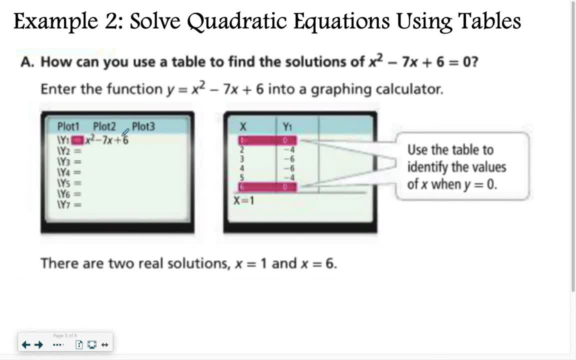 for x squared minus seven, x plus six equals zero. So when you do get these nifty little wow- I just aged myself by saying nifty- but these really great calculators in a couple of years where you can type in like x squared minus seven, x plus six.